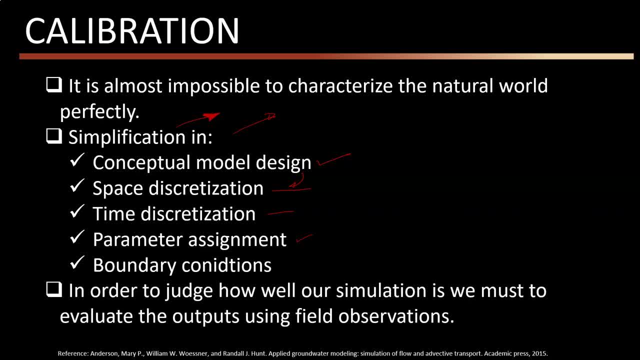 we don't have enough or too many hydraulic properties, for example hydraulic conductivity, storage coefficients and recharge information, also pumping information. so well, we have. usually we have some sort of average information, both specially and temporarily. okay, so there are. so for example, about the hydraulic conductivity we said that we usually have. 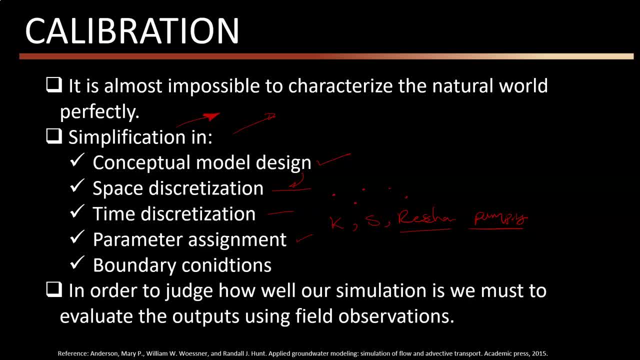 a few field measurements and we have to assign this or extend these numbers into within the entire space and again, the boundary conditions and the packages that we talked about. so these are the source of simplification of our groundwater model. so we, based on these simplification, we go and design a 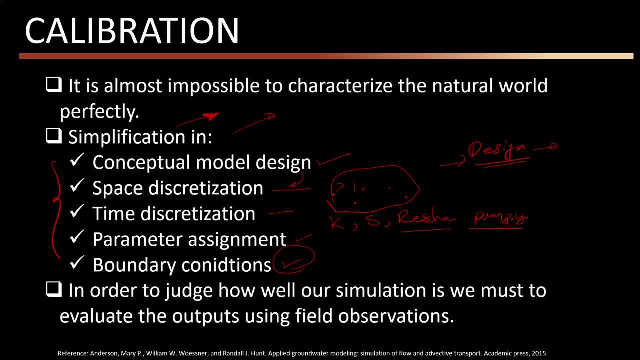 numerical model. okay, and after that we go. we want this numerical model to go and solve for H or Phi at X, Y, Z and T. all right so, and we have a tool of mod flow which can go and solve those partial differential equations and find a head at each X, Y, Z. 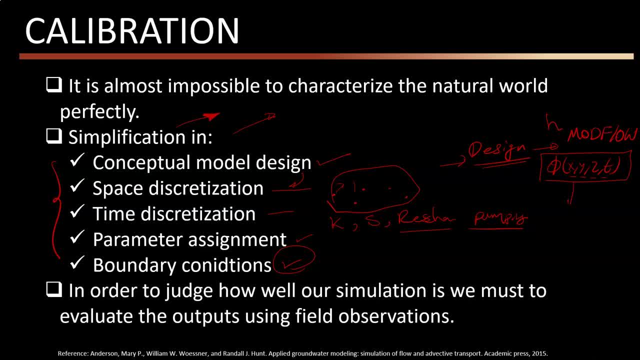 and T, but how we can go and judge how well our simulation is okay. so, technically, to estimate or to evaluate the results of our groundwater model, we have to use some field information or field observations. so, technically, you go to the field, for example, if this is your field, so you model this system, but you have some monitoring. 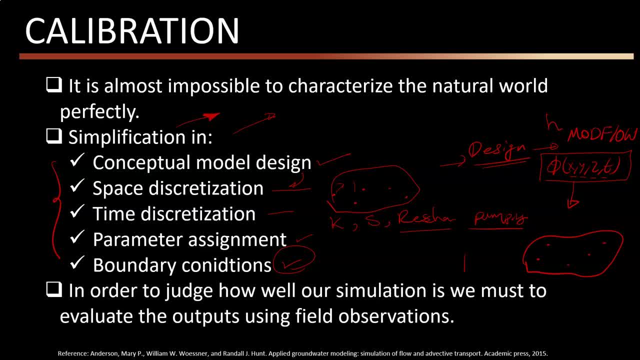 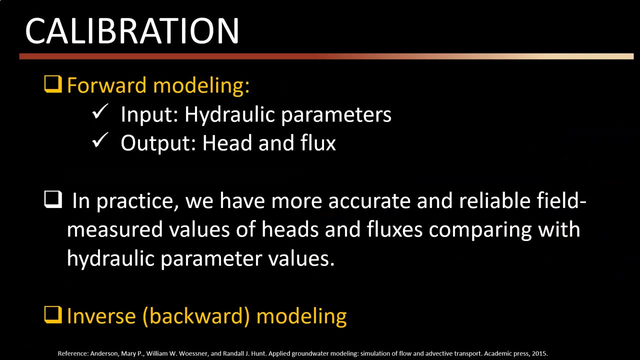 here, here and here, and you have some observation data here and you technically want to match- to see how your model simulated the head here and how you measured it in the field and based on that you judge how well your model is okay. if you remember, we divided, uh, the groundwater models. 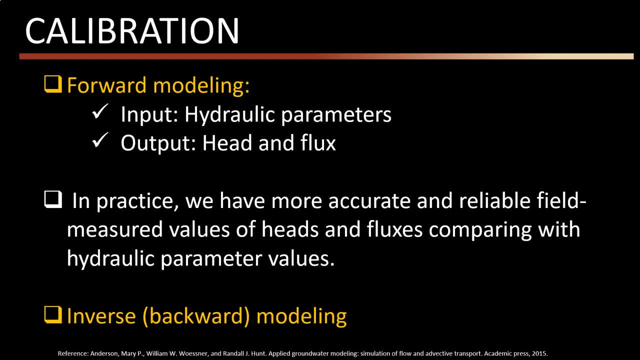 into two main groups of forward modeling, in which you input hydraulic parameters or sinking source terms and technically you go and solve for head or flux. so this is the forward form of groundwater model, but in practice we have more accurate and reliable field measured values of heads and fluxes. comparing with the hydraulic parameter values, it means that we uh. 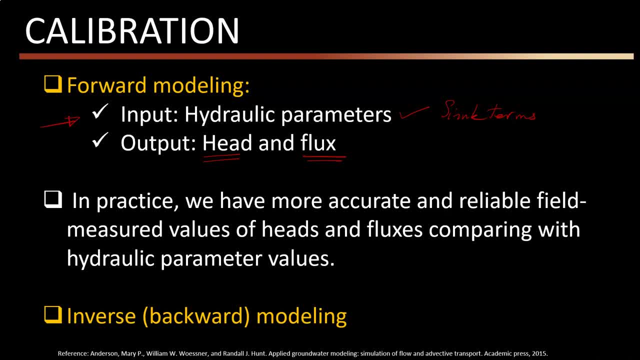 here in this part, when we input the hydraulic problem or parameters or properties into the system, there is a huge or or considerable, considerable and notable uh amount of uh inaccuracy in our parameters. so it doesn't matter during the measuring the hydraulic uh conductivity at that specific location or due to uh the extrapolation or interpolation uh processes. 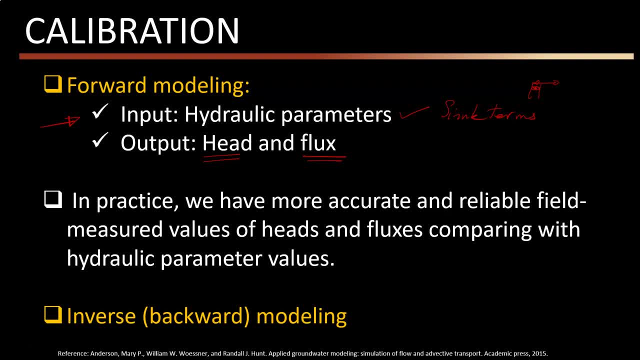 so, uh, but we can say that, uh, the groundwater head, which were measured or observed at the field, are usually much more reliable compared to the hydraulic parameters and the other properties that uh, we have here. so, because these are the usually these are point information, so you spend enough time and uh, energy, uh here, and technically you go on based on the. 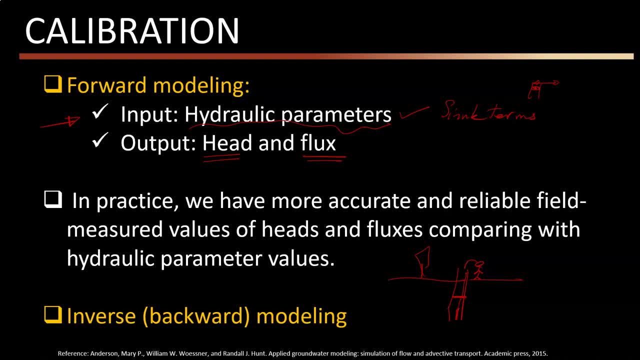 tools that we have. you can simply go and you put the transducers, or there are other multiple uh ways, but you can go and have or make a good and reliable data base of head and flux in the field. okay, so because of that, people uh proposed another form of groundwater modeling, which we called inverse or backward modeling. 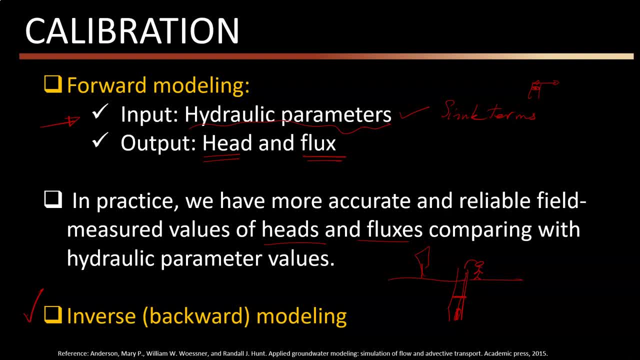 so in the backward modeling, essentially our input value. so we have uh, we have the information at the monitoring wells and we go and change the ks or uh, sinking source of values- to uh to match the observation with the simulated results. so technically now these are the unknowns, okay. 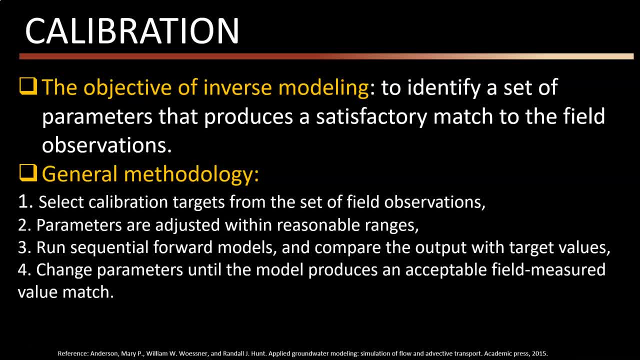 so this process, uh, the process in the inverse of modeling, is called calibration, and uh, the objective of uh calibration is to identify a set of parameters that produce produces a satisfactory match to the field observation. okay, to do that. the procedure is almost the same. so these are the main steps that 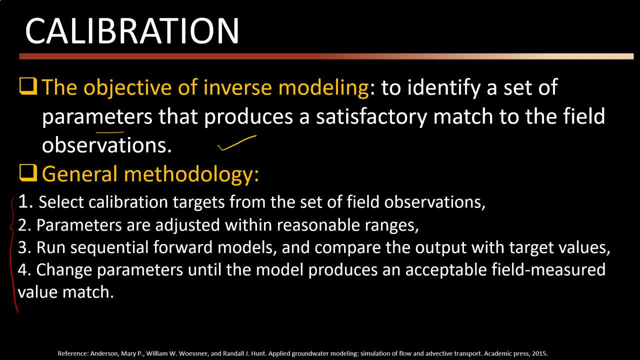 you take to inversely model your system. first you need to select some calibration targets so which are technically usually our. for example, our it is the groundwater head fluctuation information, or that might be the amount of flux or flow information into the river lake, and information like this. so you have to go and find some good calibration targets then. 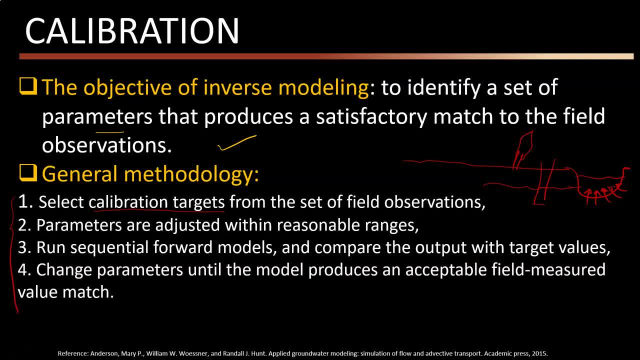 you need to think about the reasonable range of the hydraulic properties and also forcing hydrological forces like recharge, et and so on, and you need to define a reasonable range for your parameters. then you go and run a set of forward models. you run forward models, you go and find phi and then you compare your simulation with the observation. 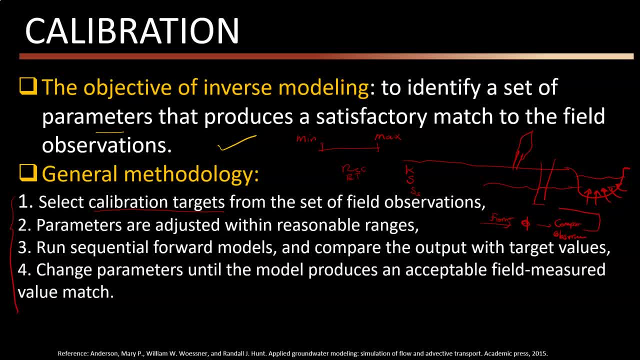 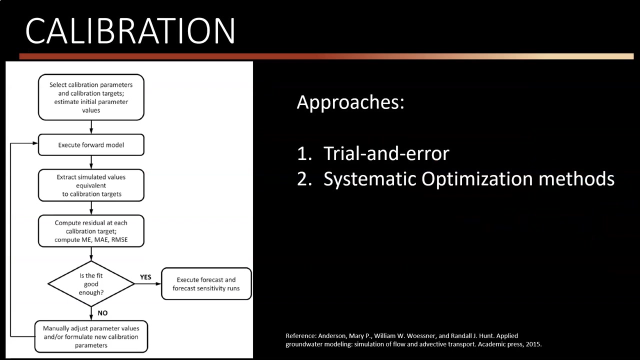 and, based on that, you correct or you change your input values and you come back and again and actually uh repeat uh this loop until you get a good um or close simulated and observed values. okay, so this is the general uh uh procedure. this flow chart shows uh a similar procedure, uh, a systematic way to go and find. 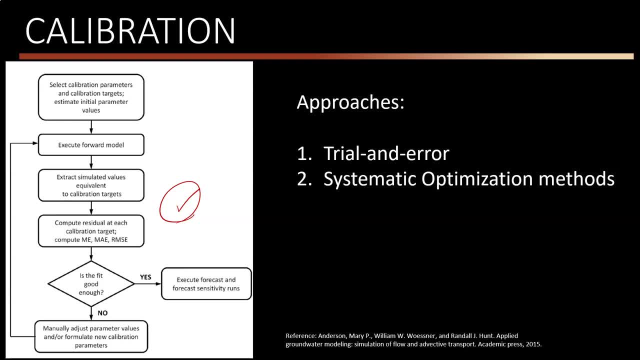 uh or calibrate the model, but uh, we can uh categorize uh the calibration methods into two groups of uh. that would be better to say manual uh trial and error. and second is the systematic optimization methods or systematic uh trial and error. so i i i think that would be a better uh. 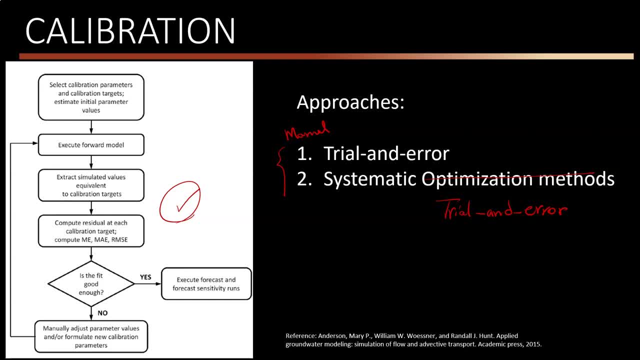 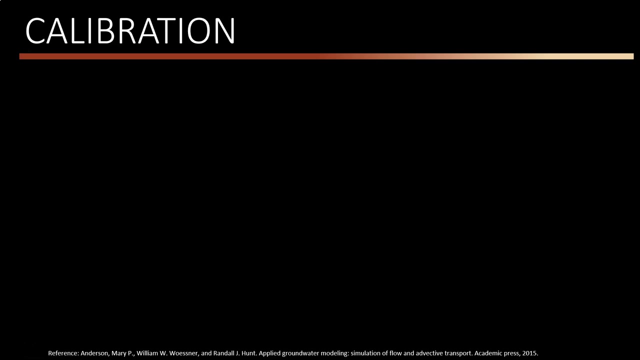 that would be better. uh labels for these uh processors. so the manual, a trial and error, and systematic trial and error or numerical trial and error, so that we are going to talk about in next slides. okay, bye, um, okay, uh, in this session i don't want to uh spend time to go and uh. 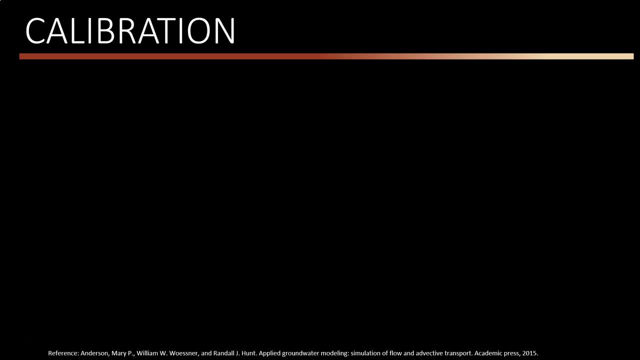 think or um talk specific to the data that we're using. so i'm going to go ahead and take a look at this this session. so if we want to go ahead and go ahead and take a look at this session, so if we want to go ahead and do some, 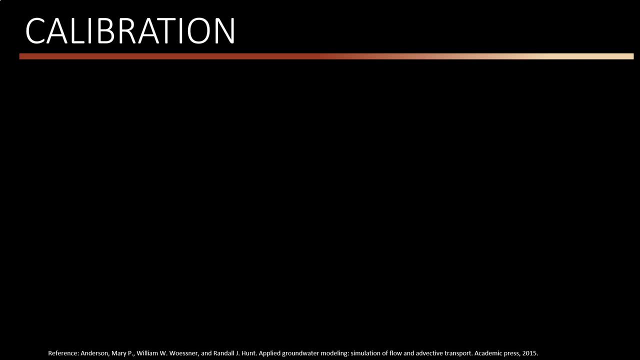 about the systematic mathematics of calibration, but what I want you to learn here is that I want you to learn why calibration is important and hard. it's how we can judge and decide that we have done a good job in calibration. so these are my main objective and goals, so we usually have very good in next slide. 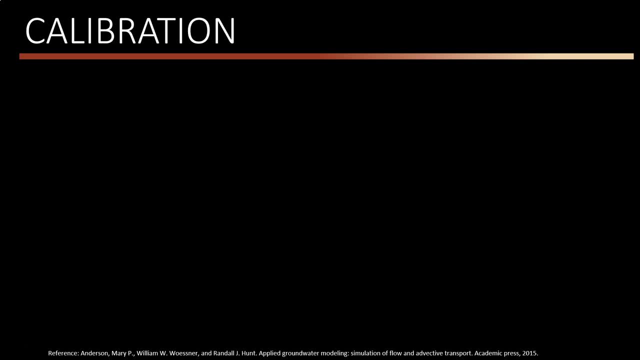 you'll see that and also you're going to practice this calibration as a homework, you'll see that there are some softwares which help us to calibrate our groundwater models and we, as a groundwater modeler, not necessarily we need to know the very advanced and complex mathematics behind the. 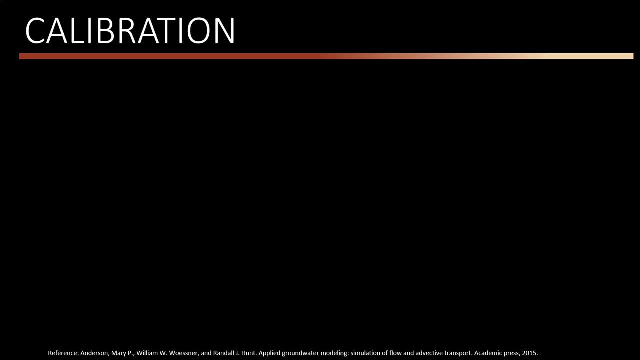 calibration methodology, but and and GUIs that we have. they have done a great job and they've created a very easy and practical interface that we can go and apply those calibration methods. so the mathematics or the calibration method is not my focus, as I said, but I 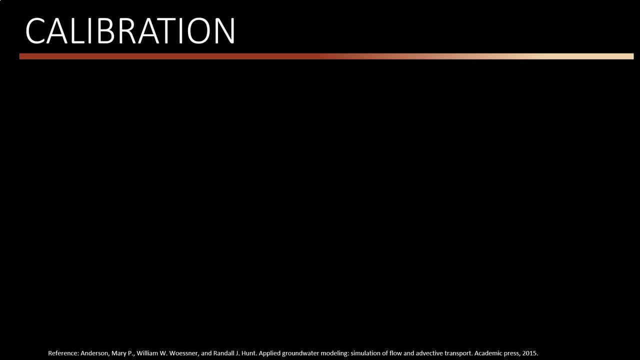 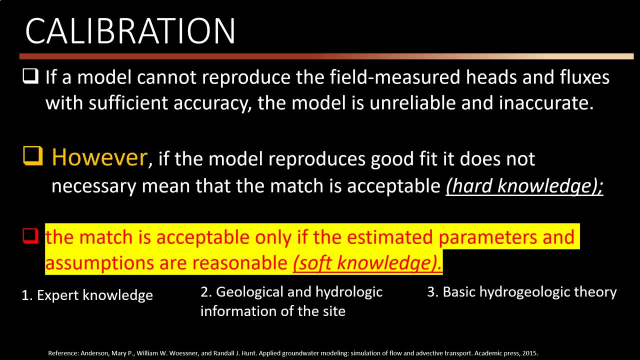 want you to know the philosophy behind the groundwater calibration more in our next slides. so here, technically, as you can guess, if, if you created a model and if your model cannot sufficiently simulate or create, defy or head information or flux information at a different location and at different times based on how they film the정diagrahia. 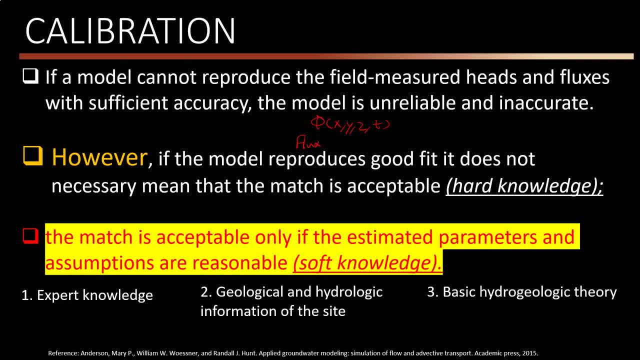 on or compared with the measured field, measured data, then you can say that this model is unreliable or inaccurate. okay, so that that that is very intuitive. however, if the model produce, even let me and. but: however, if you have a model and if you see that your model, for example, so, for example, suppose that this is the 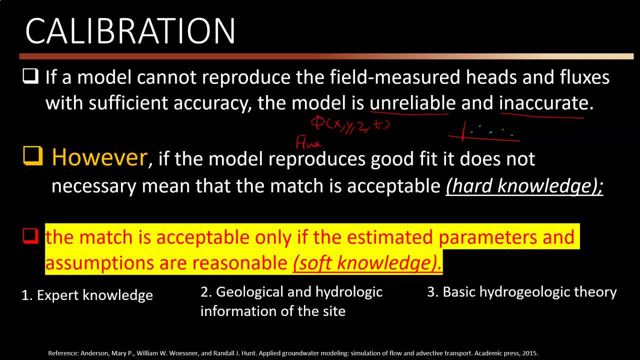 fluctuation information and your model have created very good results like this. it does not necessarily mean that it is right, or it, or it does not necessarily mean that it is a reliable and accurate model. okay, so technically, if the model produces good fit, it does not necessarily mean 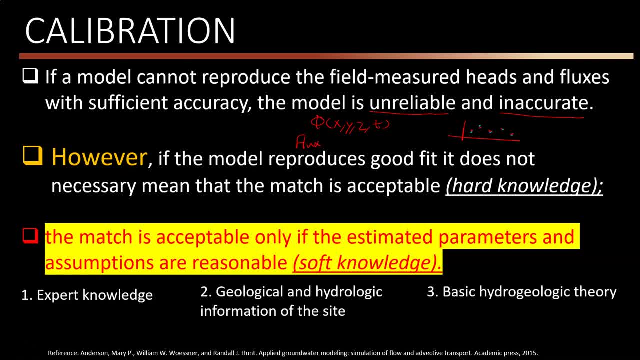 that the match is acceptable. so we call this hard knowledge, that actually this is very important thing that I want to spend time and discuss this- the match is acceptable only if the estimated parameters and assumptions are reasonable. what does it mean? we call this soft knowledge. what does it mean? it means that for 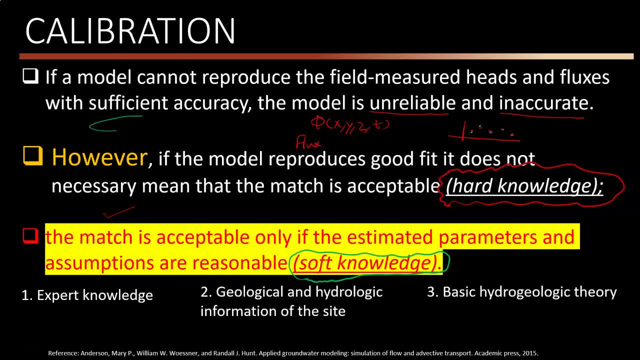 example, you go and, for example, suppose that this is your conceptual model and you have one monitoring will here and you created very good match like this. but you see that, for example, the K value here, for example, suppose that this is a sandy aquifer and you expect a relatively high hydraulic conductivity based on the 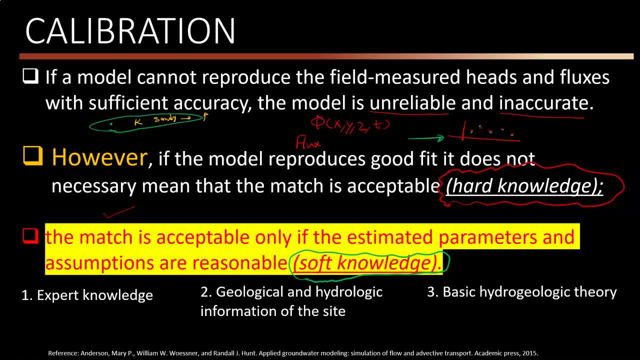 geological information that you have, but your model has created a very good fit, but the k value is so low and they are in the clay uh range. okay, so this is one example. okay, so this way, this is a soft knowledge, the geological information knowledge that you had. 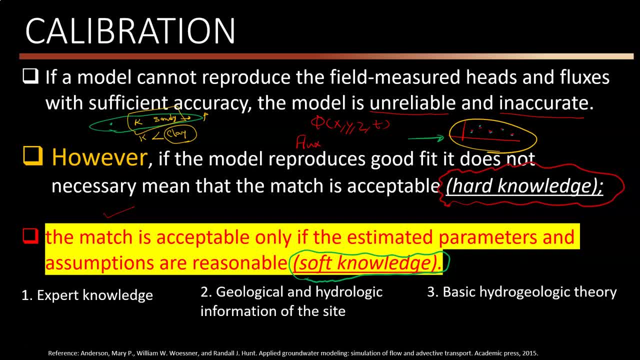 was a soft knowledge. but uh, you need to technically to do a calibration. you have to check both the hard knowledge and soft knowledge. so your model should create it reasonable and accurate enough. the head and flux information and also the calibrated values should also make sense. okay, so 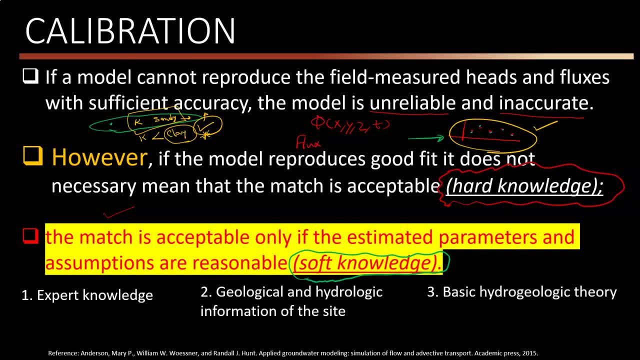 this is very important- that actually usually people uh- i've seen that actually so many uh cases which they have created a very good fit, but uh they didn't think or they didn't uh uh discuss the uh the soft knowledge part or the uh additional information that we have. 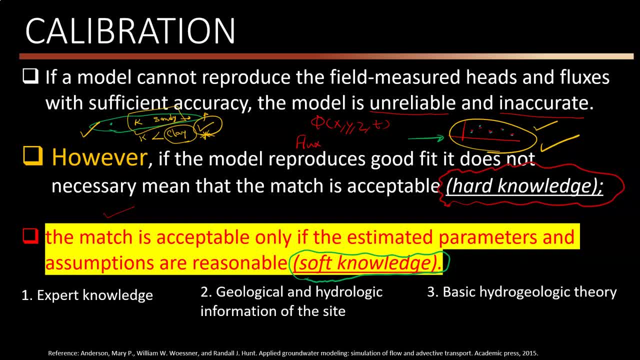 that actually we want our model match with those information as well. okay, that would be hydraulic property. that would be, for example, the flux information under a piece of uh or section of river or lake, and or pumping rate, recharge rate, uh, such information, okay. so essentially you need: 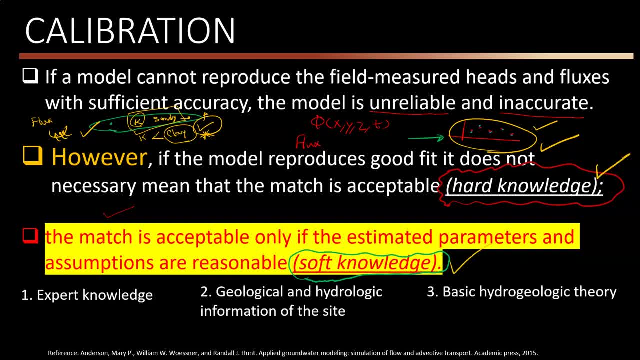 to check both hard and soft knowledge. but uh, checking this part is uh not usually very easy. so you have to have a very good expert knowledge. you have to have a very good geological and hydrological information from the site which you can go and find from the report, uh reports, uh papers, and also you can talk. 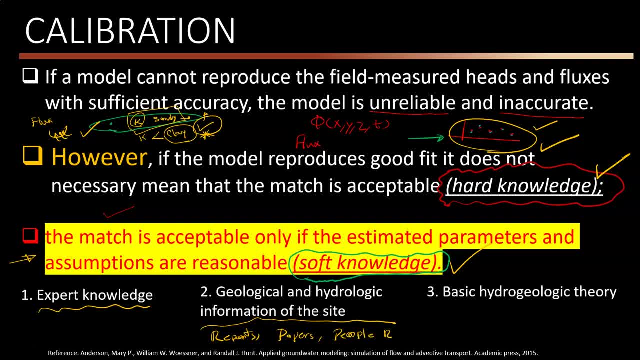 with uh, uh people and uh, researchers. okay so, uh, and also, you have to have a basic hydrological logical theory, or you need to know the basics of the hydraulics. okay, so, for example, if you are, for example, you, if you have an information of flux, or 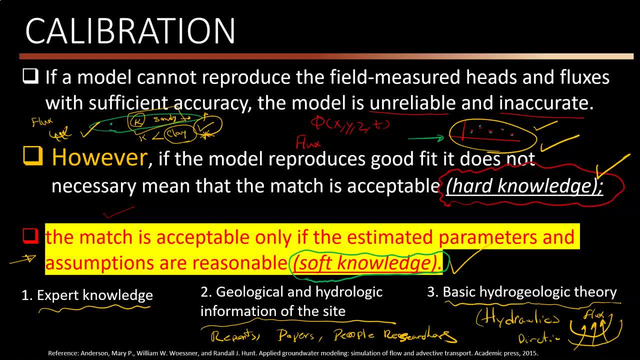 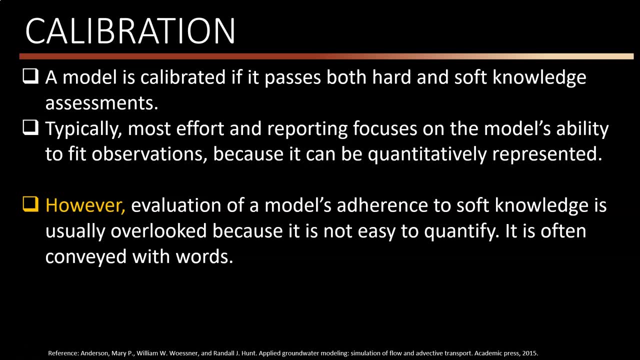 velocity directions and so on. so you need to actually check your model to see that actually it is hydraulically sound. as I said, the model is calibrated if it passes both hard and soft knowledge assessments. typically most effort and reporting focuses on the models ability to fit observation, because you can go. 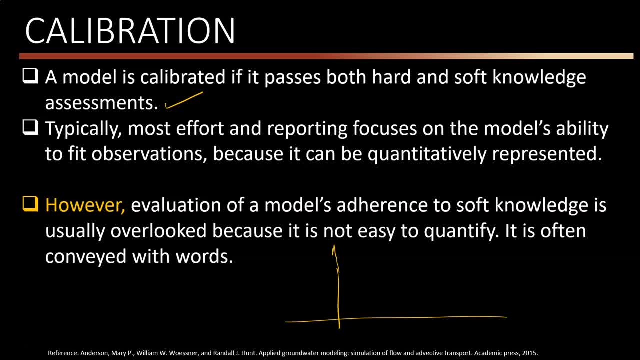 and quantitative- or visually or quantitatively- show the fit. so if you go and see the papers, they usually they have done a very good job on feeling the data, but they have a very weak and incomplete discussion on the evaluation of models. adherence to soft knowledge is something which is lacked. 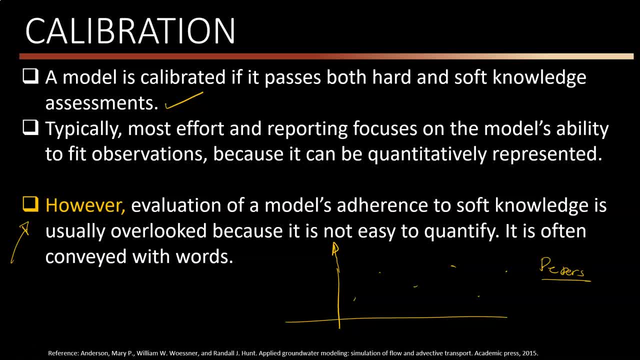 usually in those reports and the problem is that usually it is difficult to go and quantitatively show or represents the soft knowledge matches. but, and you know I mean there's no way you can. you need to go and you can vary the matches in the soft knowledge part just by verbally describing the system and 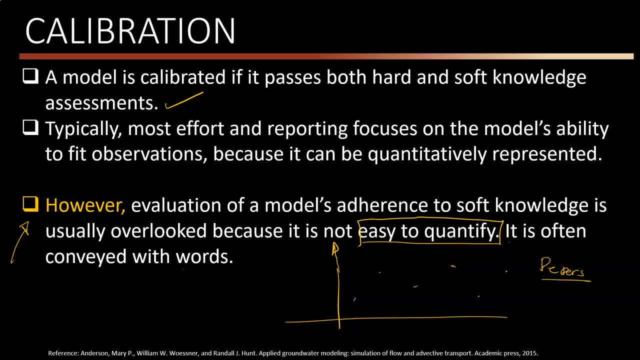 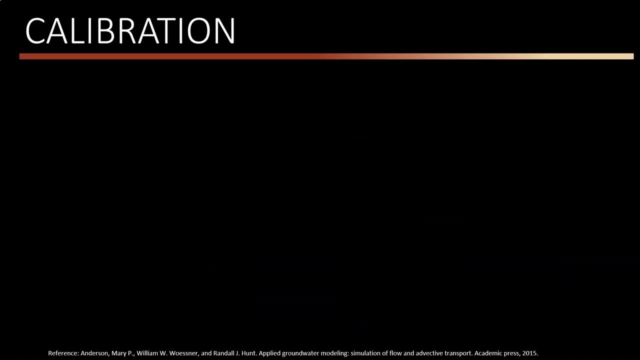 describing the structures that the, the systems run under. yes, so it's not that it's just beating the self-knowledge information and say that actually our model matches and consistent with these information. so here, and I want to- I want you to learn or think again about the basics or philosophy of groundwater modeling and 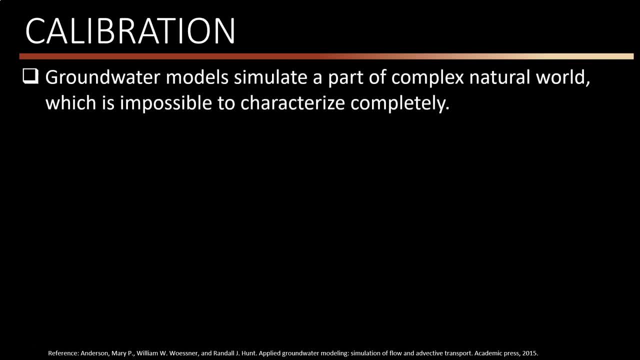 groundwater calibration. as you know, groundwater models simulate a part of complex natural world which is impossible to characterize completely. so it is almost impossible. you go and measure the hydraulic conductivity everywhere, it doesn't matter. even in very small laboratory scale problems. we have difficulty to go and find a very proper and accurate, especially in 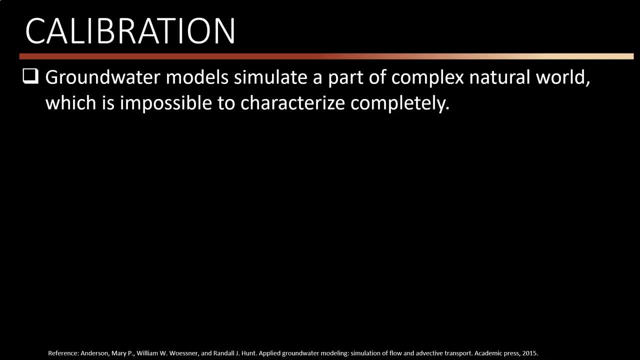 temporal distributed information in the big scale and field escape problems. definitely this problem is much more worse. so so we can say that they feel the scale groundwater model is always a simplification of the true hydrologic system. so the simplification is the word that I want you to think actually to. 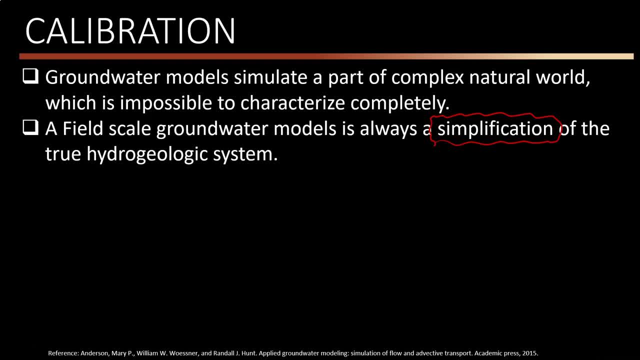 this exceptions the fault features of a few models. you might have seen thetheming of everything was completely simulated for a certaincient of water samples. it doesn't have something really to do with rock technology. so what we're struggling with is: how can we do more, how to communicate with the world? 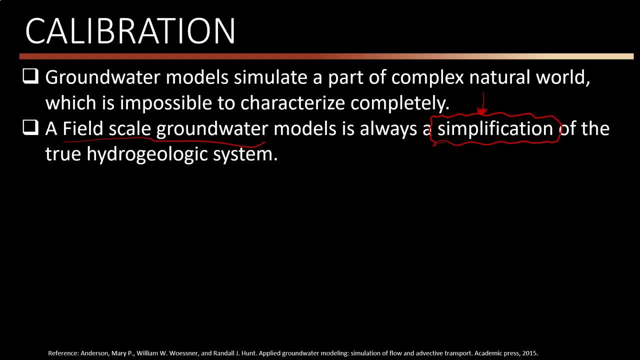 evidence. so we want to now to come back to fields escape, groundwater models, but from the laboratory, small scale. laboratory scales, because in the laboratory scale, since it is a smaller problem, you as a modeler have a control and we ourselves. we go and set up our laboratory model, so we go and create specific k values, s values and so on, and we have a better 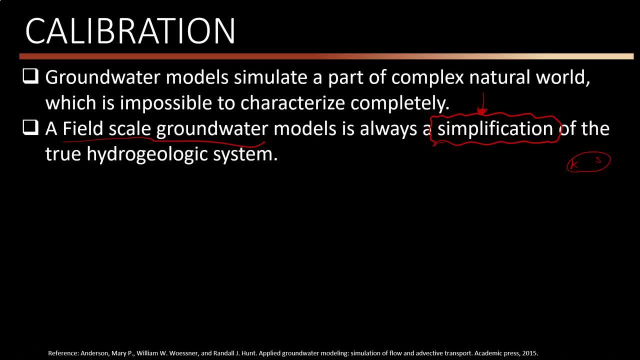 control on the system. that's why the level of simplification and groundwater mod, the laboratory scale and small scale models is maybe less but still there is some sort of simplification during those types of studies. so in the field situation we usually- and you or me I may say that always- have more unknown parameter values than known. 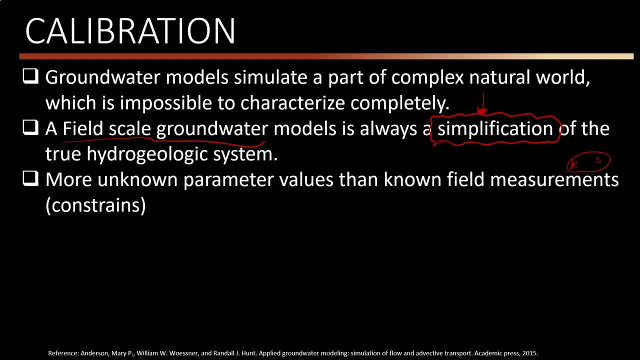 field measurements. okay, so if you go, if you think about this, the measurements that we have a mathematically they are actually our constraints. that you will see later actually what I mean by constraints, but usually we have a very few. for example, we have only five monetary. 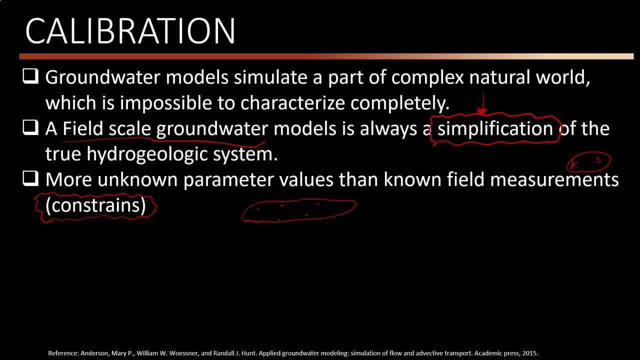 wills within, for example, a five kilometer, one kilometer problem, or we may have just very few k values here and here and here, but technically the k values in other points are unknown right. so so this is technically. we would like to go and create and find the k values. 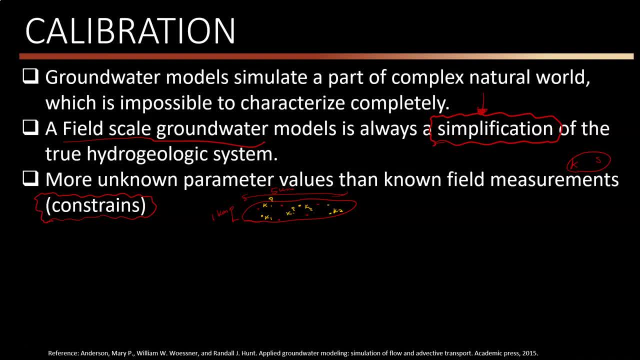 for example everywhere, and compare them with the measured k 2 and based on this, actually, we proceed calibration process. okay, so we usually have very limited and few known and observed values, which cause a problem and also the inverse problem and because of this, the inverse problem, you. 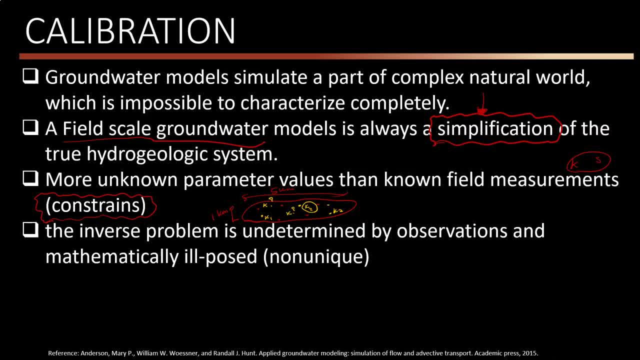 are technically undetermined by observation and we call them mathematically ill-posed. So the mathematically ill-posed problem means that since you have very limited constraints or known values, technically there is no unique solution for your problem. It means that there 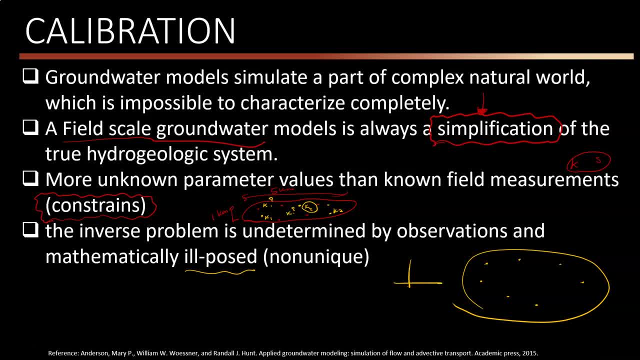 is a group of solutions which can go and create a very good match, for example, if this is the observation and simulated at this point, okay, So there are multiple scenarios of the distributed k values or s values here which can go and create a reasonable and close simulation. That's why 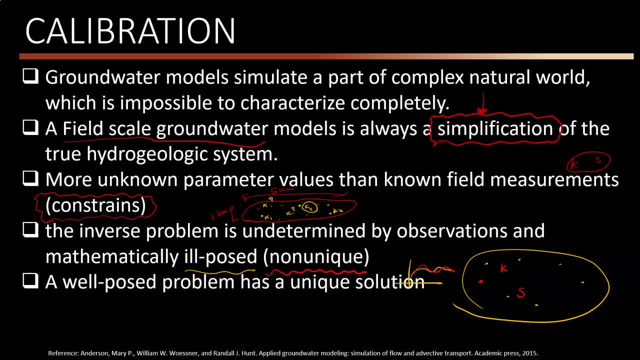 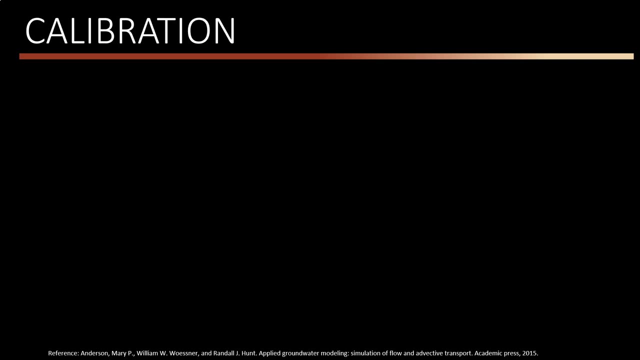 our groundwater model is so important. The two models are inherently ill-posed or they suffer from non-uniqueness. okay, But there are some ways that actually we can address this problem. So how we can address the non-uniqueness issue First. first, we, as graduates, we are using linear simulation, which is a very useful 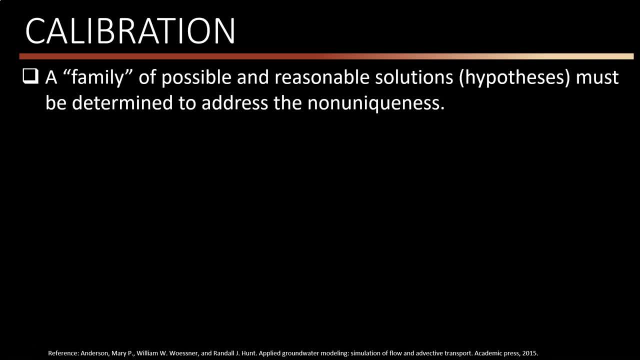 water model, we need to go and identify a family of possible and reasonable solutions for our model, which herein I call them hypothesis. so we have a group of hypothesis, like I identify, five different models and calibrated results, which creates a reasonable match with our observation and also with soft knowledge. okay, so remember, we have to check both hard knowledge and soft knowledge, both. 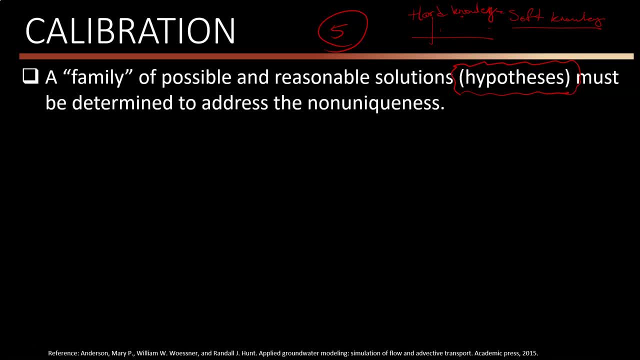 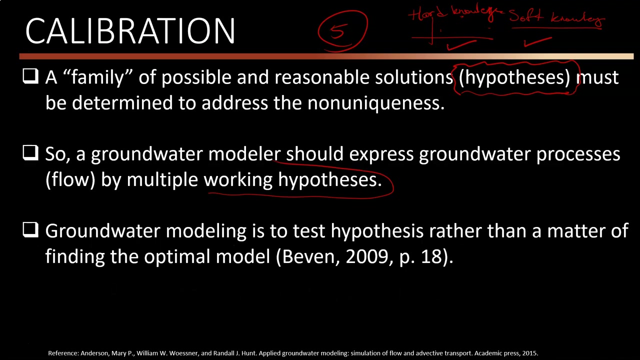 so we have five hypotheses. which passes the tests then? so groundwater modeler should technically express the groundwater processes, which are the groundwater flow information, the velocity direction, by multiple working hypothesis. okay, so groundwater modeling is. can be said that essentially the main objective of groundwater modeling is to go and test hypothesis. 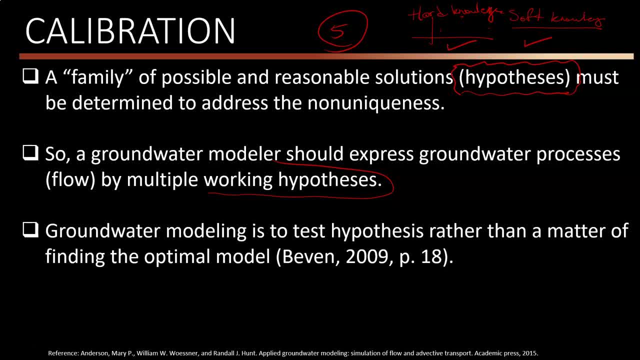 rather than a matter of finding the optimal model. so it is much more reasonable and it is much more defensible and accurate if we go and find a group of hypothesis which are usually- they are not too uh actually from each other, but they may- some of them may have, for example, uh have- better results. 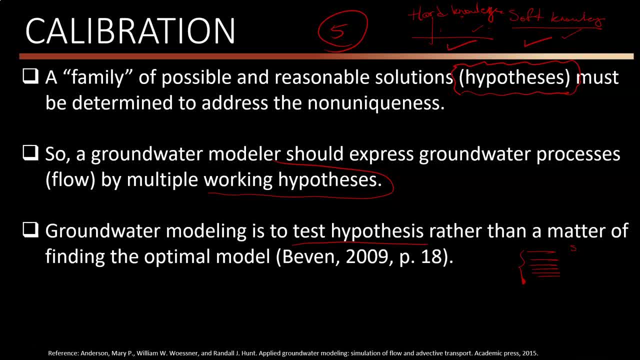 once we test the soft knowledge and hard knowledge information. but it is good to represent the system using a group of uh hypothesis or we can go and uh discuss the other models and hypotheses which are out of uh this group, which is important. so there's a very 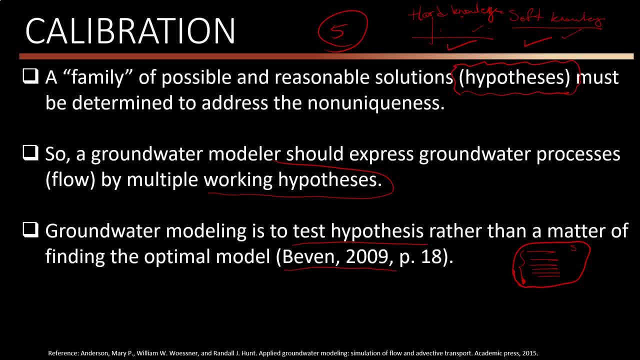 nice discussion on the Beaven uh paper published in 2009. if you're interested, you can go and read uh the philosophy of uh the groundwater modeling, but in practice, once you sign the contract, your know the what the software tries to do with this part um. so therefore, this is: 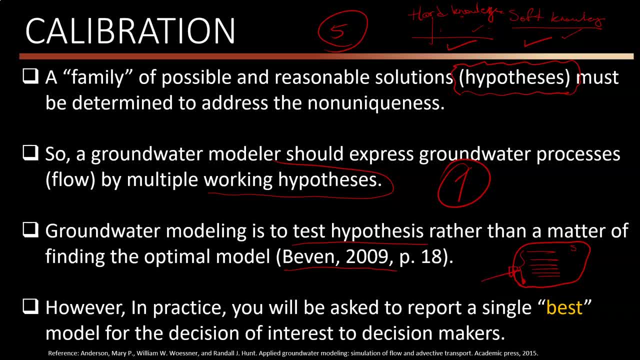 a tool that can be used as a guide to chickens how they're connected. uh, perhaps we've already correct, but it could be used as a tool for like kinds of uh. uh, all these experiment and experiments which we, as twentieth-century, know. you can do uh from all maps at once. it's very easy when we understand. 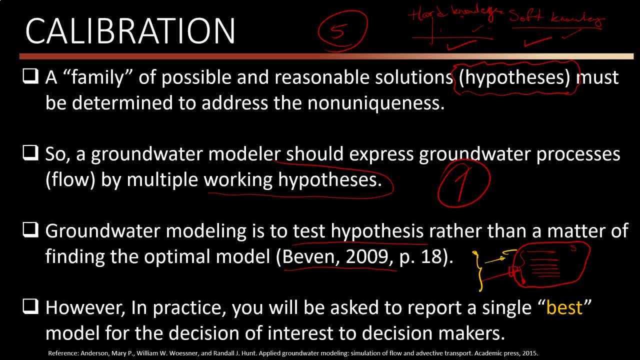 us to go and directly go and find the best options. okay, so uh they, they usually don't understand uh the system and and i think this is part of our uh responsibilities as groundwater models to go and change uh this uh viewpoints uh to uh groundwater models. but anyway, so you are usually. 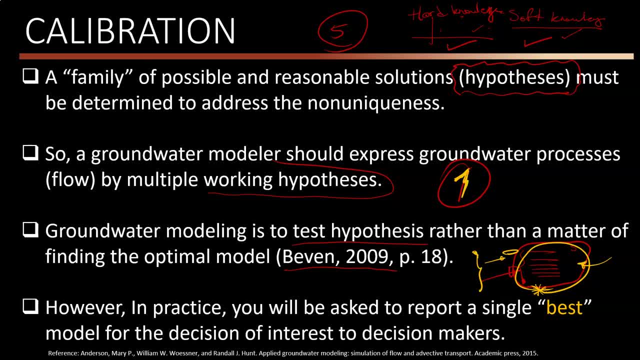 uh ask: or you're supposed to submit one solution to your uh problem, and what is that? that solution is actually the best solution which you can go and pick and you can find from the group of uh solutions that you have. okay, but how you can do that we are going to talk about this. next slides. 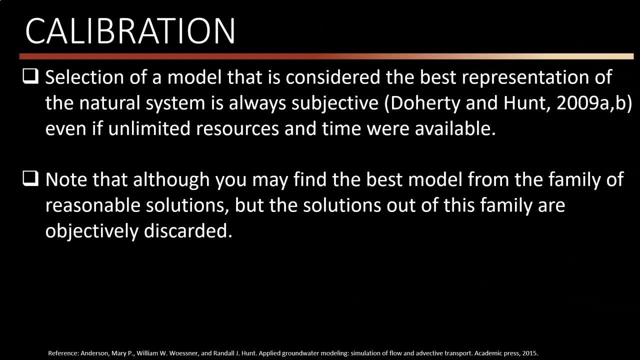 okay, so we're going to talk about this next. slides doherty and hunt. uh has explained the situation perfectly from my viewpoint. they say that the selection of model that is considered the best representation of the natural system is always subjective. so it is always subjective, even if unlimited resources and time were available. so 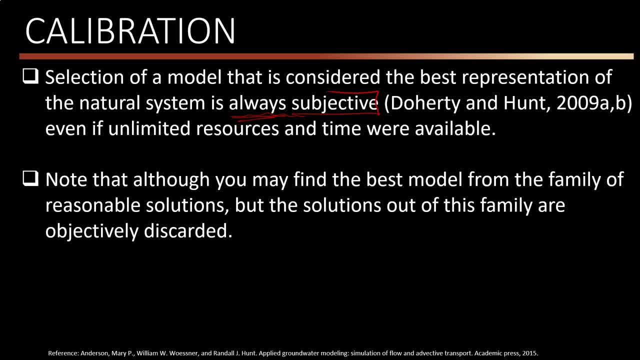 uh, what they want to say that? they want to say that finding the best representation of, or the best solution to, so many different things, like the objectives of the modeling, a modeler itself or, in some points, maybe, the client or decision makers that you are working on, it may depend on the amount of time. 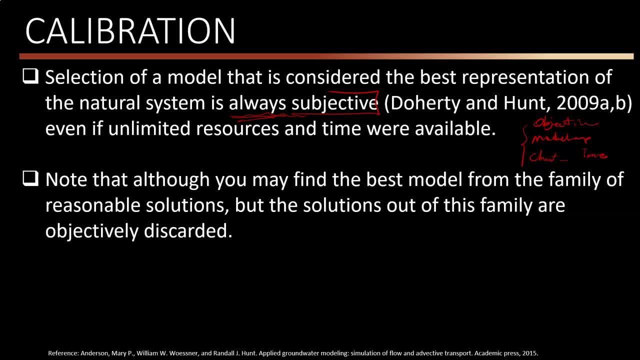 that you have for modeling or an amount of funds that you have to do this. but what you need to know and learn is that always finding the best calibrated model is subjective, and that's why the experience and knowledge, or gains knowledge, is something which is very important in groundwater modeling. it is 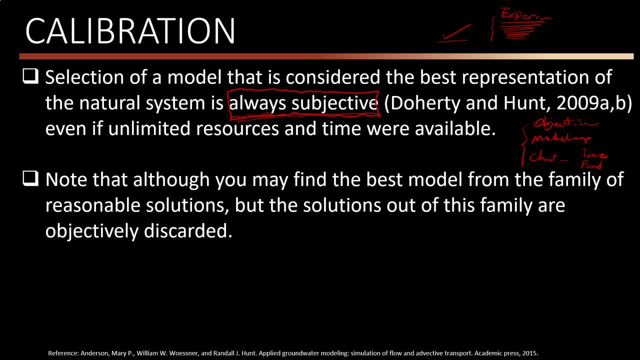 like it's actually. it is like an art. so you need to experience, you need to learn the tricks to become a good groundwater modelers. but it is very, very important to pay attention to this fact that, although you may find the best model from the family of reasonable solutions that you have determined, but you need to and and 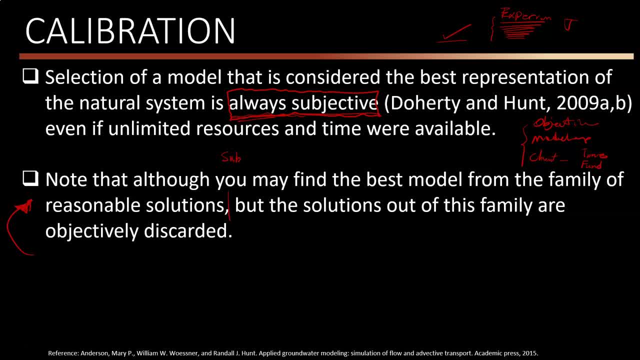 this process is subjective. okay, so you subjectively go and, based on these information and based on your experiences, you go and find, for example of five hypotheses or five solutions, okay, which you think that they go. they all pass, excuse me, they pass both, both soft and hard knowledge. okay, but you 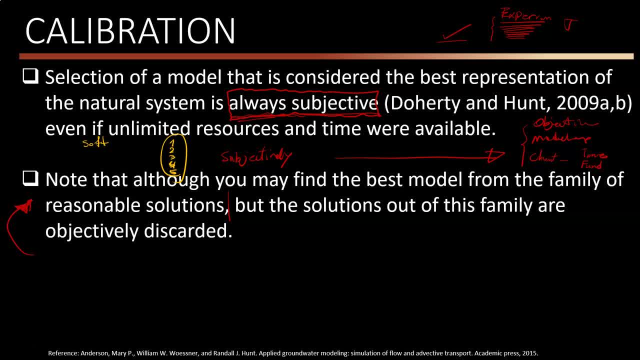 need to pay attention that the solutions, the hypothesis out of this family is are objectively discarded. okay, so technically you have objectively check the soft knowledge or hard knowledge and you you said that these hypotheses they can not be true. so there are so many other hypothesis that you can go and. 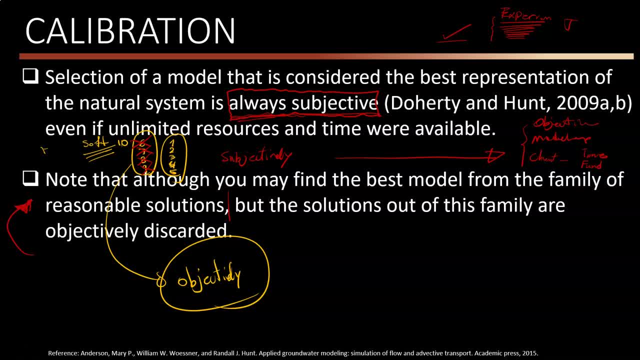 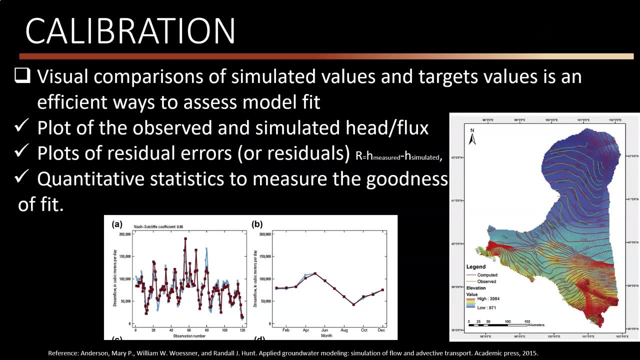 this process of is an objective process, okay, so, which is very important, and then at that is the main goal of groundwater modeling. in so many cases, there are multiple ways to go and represents the goodness of your model, or to go and decide, or pick the best solution out of. 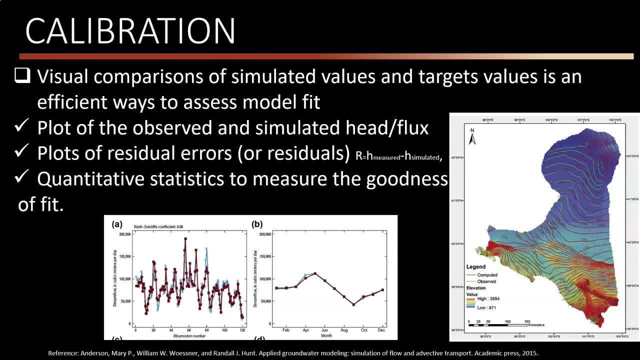 the family. one way is that you can go and visually plot the observed and simulated head and flocks data. so there are multiple ways and this is why the next slides. I've shown you some examples. for example, in this map you see that actually there are different contours. ones is red, the one 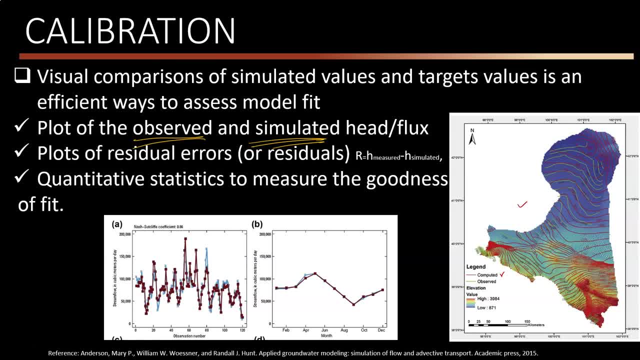 is the computed and the green is observed. so based on this visualization, you can go and find the best solution. for example, if this is the main area of your interest, you can focus on and, based on that, find the best solution, for example. or you can go and plot the observation and simulated results in a 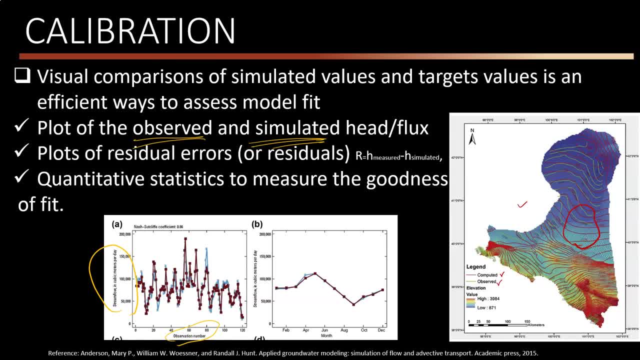 specific location and actually plot them and based on this you can go and actually compare the goodness of your simulated results and calibrated results. the other way is that you can go and plot the residual errors. so the residual errors is, by definition, is the difference between the measured and observed. so this is another. 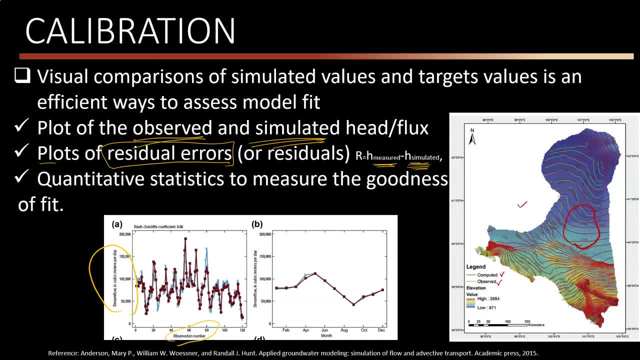 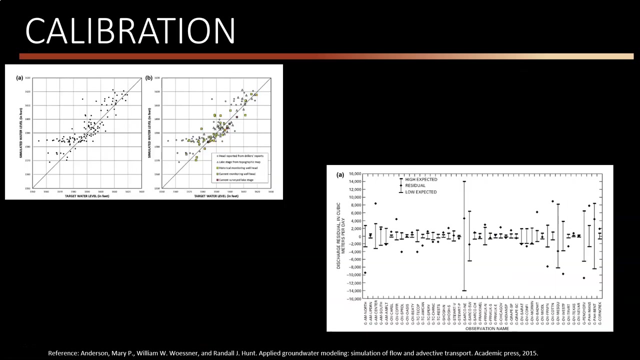 way that actually you can go and represent your results or you can use quantitative statics to measure the goodness of fit, for example, mean square errors and different form of forms of errors- that actually you can go and use them and statistically and quantitatively show the goodness of your simulation. in this picture you see how you can. 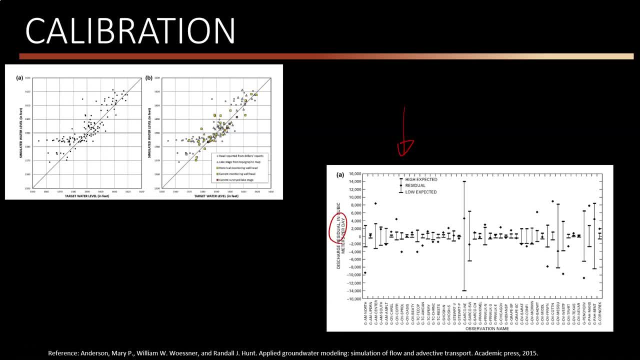 represent the residual errors and uh show the actually the the high expected and low expected values and actually compare your results or discuss the goodness of your model using this type of information. or you can go and plot the target values versus the simulated values and create a plots like this and discuss the goodness of your model. 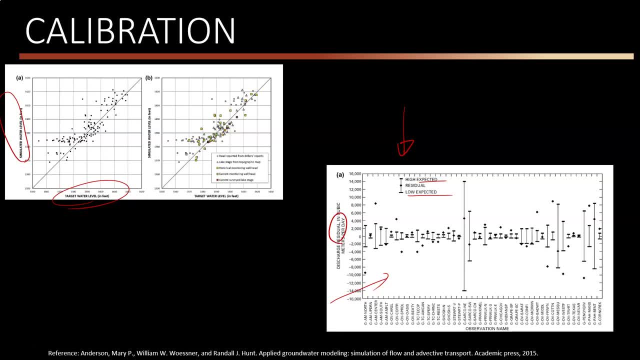 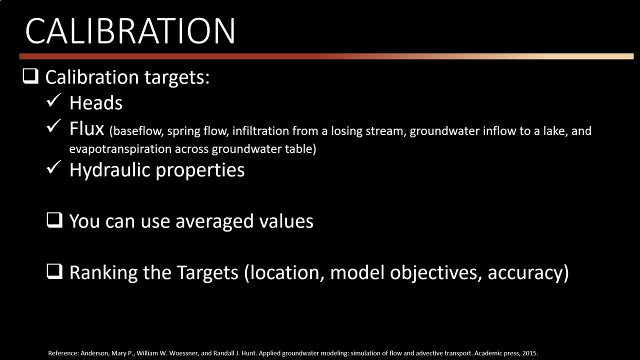 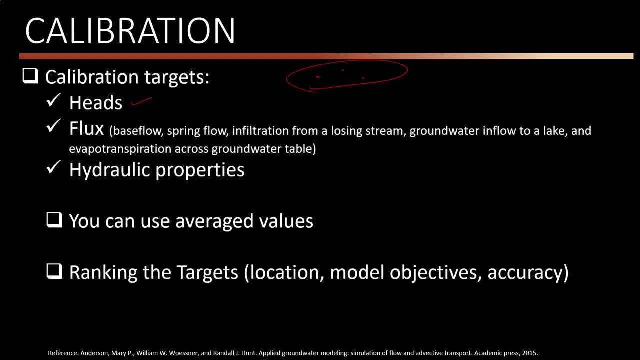 One is the head information, which technically comes from the monitoring wells, The flux information, which comes usually from different and independent studies and measurements, And also the hydraulic properties are. for example, you can set a range of K values or S values for a specific location. 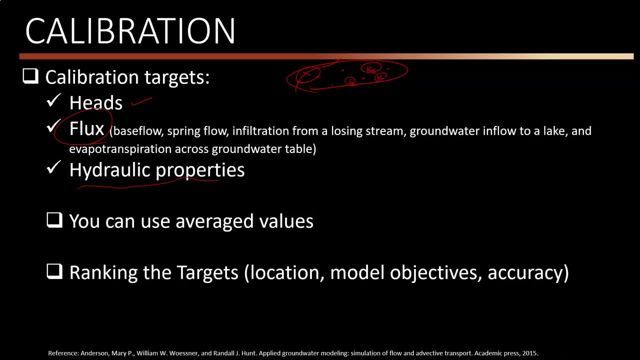 And you can use them as your calibration targets. But specifically speaking for heads and flux, and maybe in some cases that might be the hydraulic- Yeah, I mean actually, if you think about the recharge and ET terms, so you know that these values, like groundwater table, it fluctuates and it changes with time. 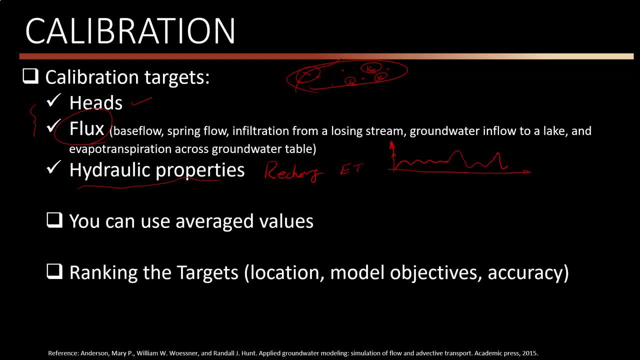 It's seasonally And in some case maybe daily. So we usually it is very difficult to go and use all of these information for the calibration, So technically we can go and again use an average data or average information to go and better calibrate our models. 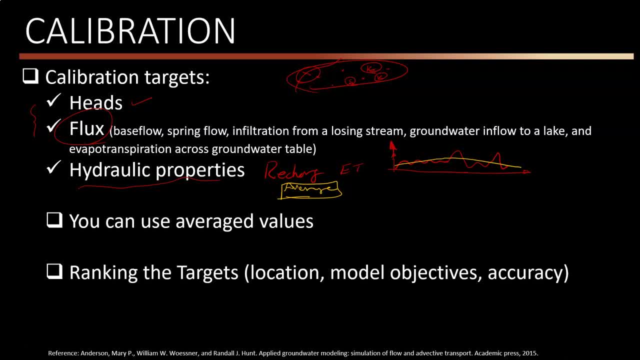 But it is. It's very important to know that You have to to have a good and reasonable I calibration And a reasonable to create a reasonable groundwater model. You need to rank your target values. So, for example, that would happen. You need to think about the location of your target values. 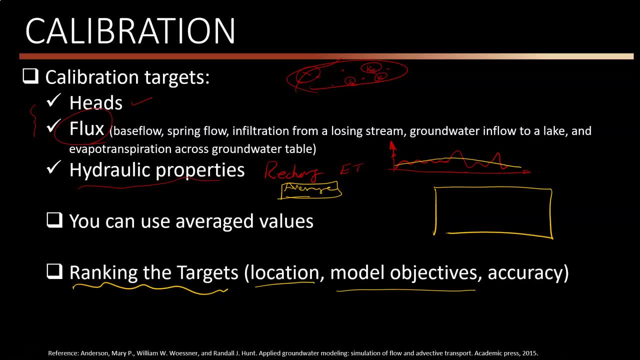 You need to think about the objectives of your model And also you need to think about the accuracy of the measured values. you know that I mean, for example, we said that, for example, if you want to go and find K values, so there are multiple ways. for example, you can use a slog test or you can use the pump test. 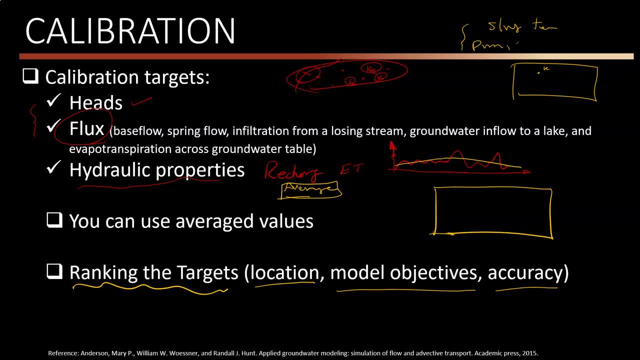 okay, each of these have their own, has their own limitations and approximations. okay, so they are not accurate and also, in the human error can play a role here and can create actually an error in our estimation. so these are the things that actually we need to think about. but, for example, if there is a factor here that we 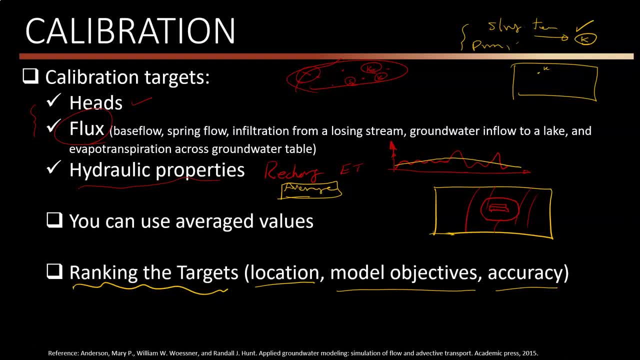 want to know how the groundwater is moving beneath this or how the contaminants which would move by the groundwater models. so technically, we can say that if you have monitoring wells here and here and here, maybe we can say that I don't know. this is just a suggestion. I would say that, for example, I can rank these as the: 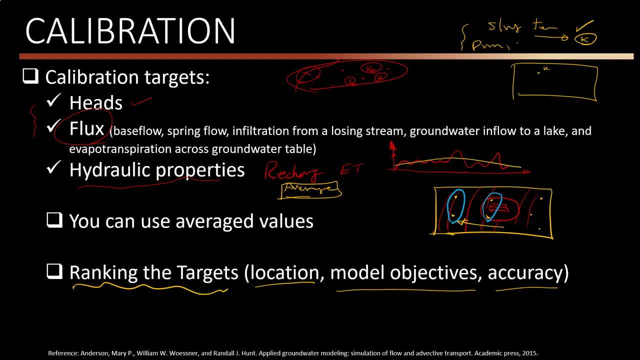 most important- and this is the second important and the upstream is the least important- points. okay, so then, if I have a family of solutions, I will go and focus on these targets. okay, and that would be. again, I need to think about that would be, for example- this is just a location example- 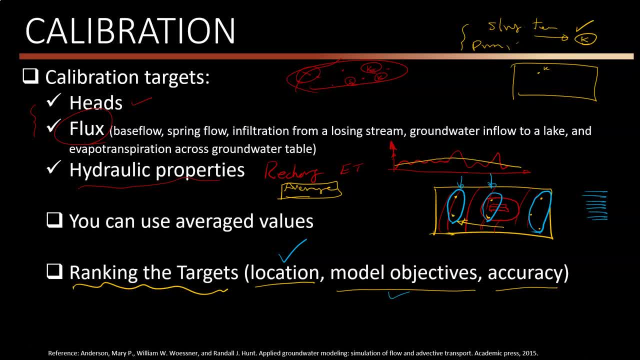 okay, so you need to think about so again, based on the objectives. I said that the contaminant transport was an object. that's why, actually, I I said that the upstream may not be very important, but so the so these are the things that you need to go and think about. so, technically, you need to go and rank. 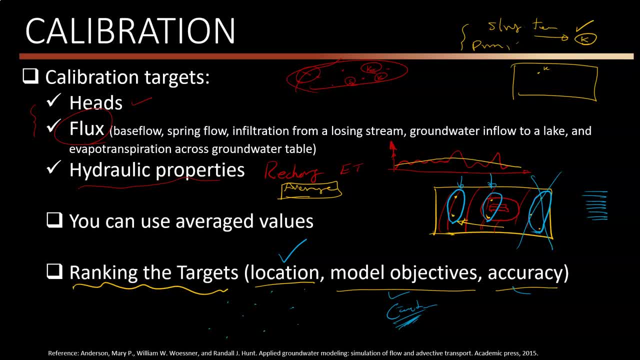 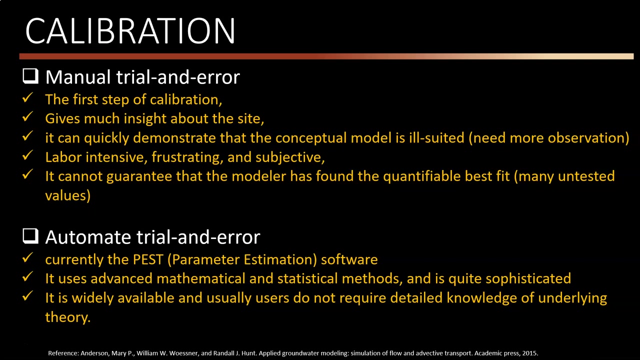 your target values and constraints and if you see that actually it is better to ignore or discard some calibration points it is, you can go ahead and actually do that. okay, we said that there are two groups of, there are two methods to do the calibration. first is the manual trial and 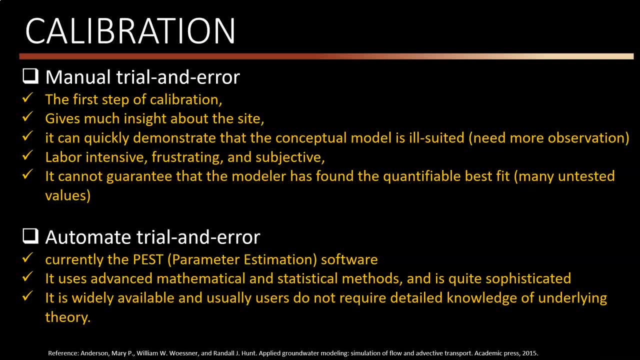 error. the second one is the ultimate trial and error. okay, so the processes are kind of the same, but the difference is that here in you have to do the iterations manually, but here there is a systematic way and software which uses a very advanced mathematical and statistical uh. 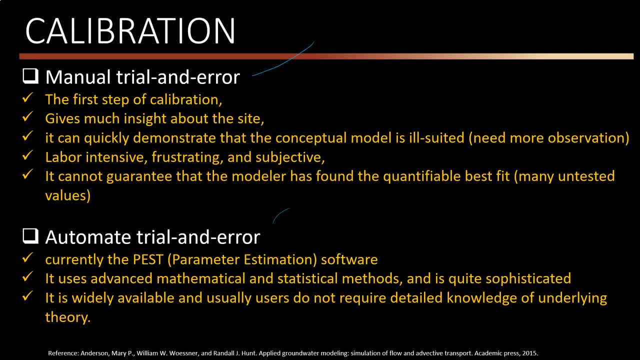 calculations and considerations and it goes and creates uh- or solve our calibration uh- models. but uh, there are a few things that I want you to pay attention to and uh think about. uh, it is very important that, although you usually will be required to go and use an automate, 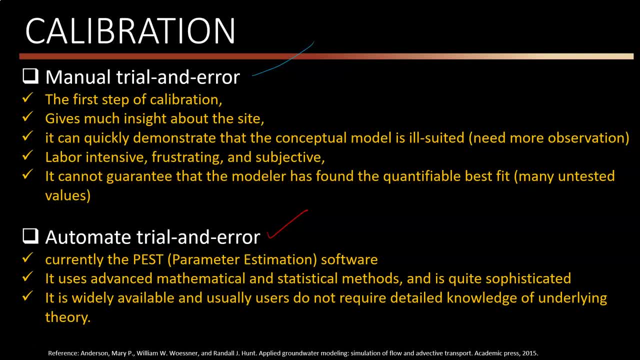 or general manual manual trial and error method, uh, or a trial and error or normal standard trial and error method. but before starting this, you uh should go and manually try to uh do the calibration and play with your model, because by doing so you will see that actually you will gain a lot of useful uh insight about the 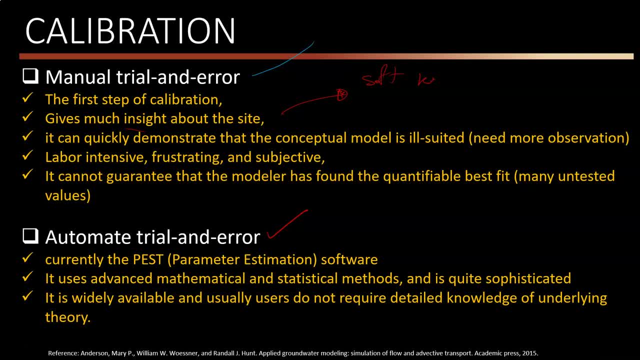 can help you in soft knowledge assessments. Okay, so technically you need to go and play with the parameters and do the calibration manually and see actually how the results change and how your system works. The manual trial and error can quickly demonstrate that the conceptual model 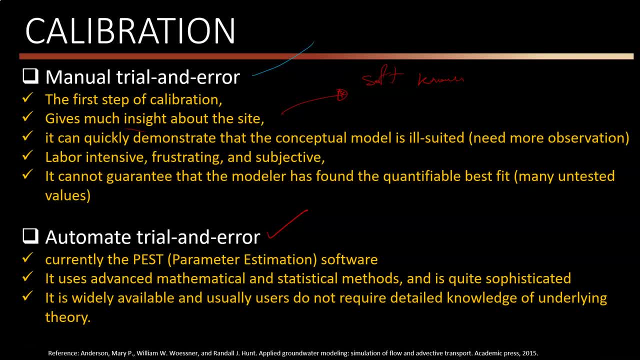 is ill-situated. So if you see, if you do the manual, if you do the trial and error manually and if there is a significant problem with your conceptual model, it will go and show you. But if you miss this process and if you directly go here, it is very difficult because these are very 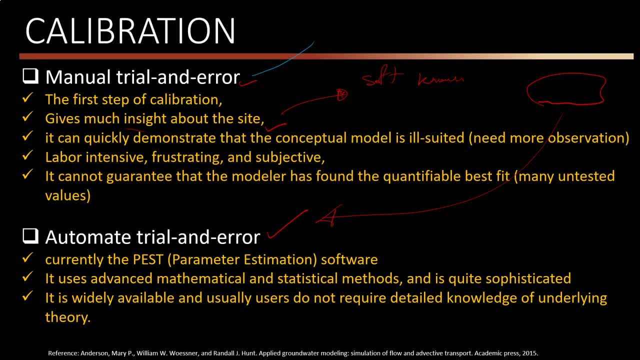 time-consuming and there are so many details that you need to be taking care of which may distract you or it may take your time and it might be too late to realize that you need to go and revise your conceptual models. But the trial and error method. 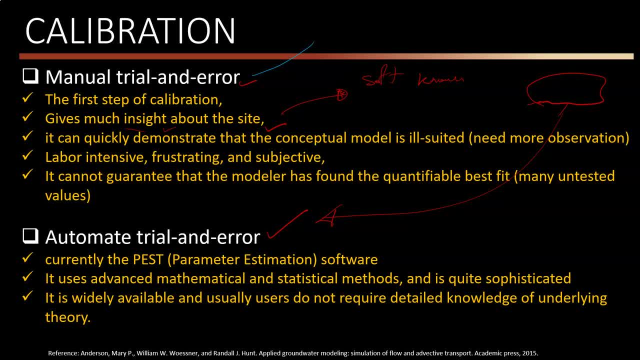 is easier, it is faster and it is much under control of the modeler. That's why it creates very good information and insights about the model. So, as you can guess, it is intensive, it is frustrating and it is very subjective, So you need to be very patient You. 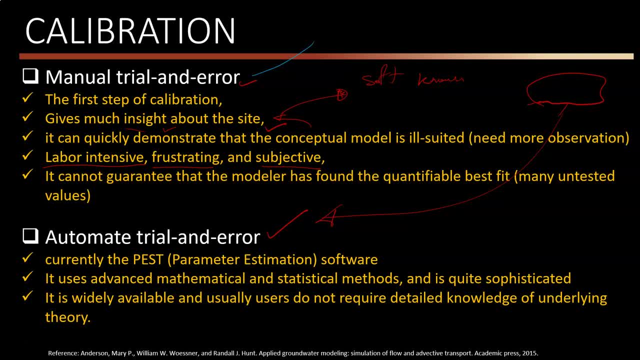 need to know that before starting this, you need to know that it's a very frustrating process and you need to actually do a trial and error a lot of times. But you need to know that this method cannot guarantee that the modeler has found the quantifiable best fit for your solution. It means 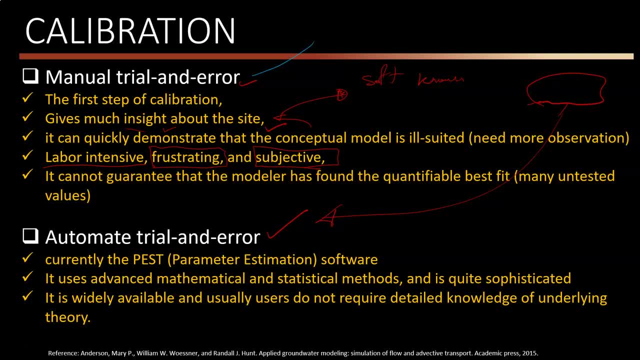 that there might be many untested values, that you didn't have time or for some reasons you couldn't go and test and try them. So this is the big drawback or the big limitation of this, the calibration. But you don't have this problem, or you have a very less impact here in the 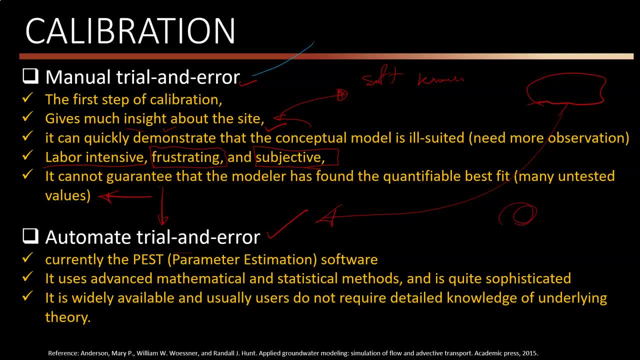 systematic trial and error because it goes and iterates your calculations a lot of times and it itself goes and tries to go and find the best hypothesis and best scenarios that focus itself to that area. Now in groundwater model world we use- we usually extensively use- the calibration software known as 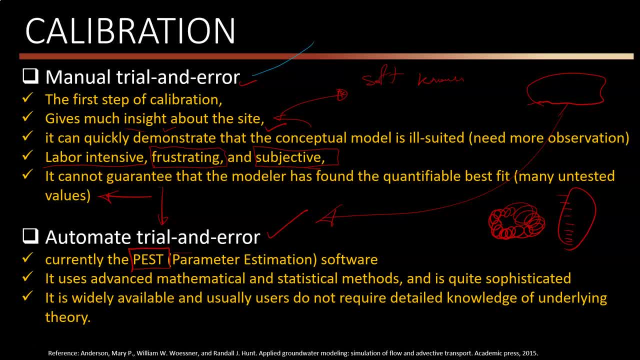 PEST, which stands for parameter estimation software. It is developed by John Doherty. John Doherty has done a great job here. He spends a life actually- and he created- I think it might be, if I'm not wrong, it is a 30 years efforts of John Doherty to create a very advanced and sophisticated model. 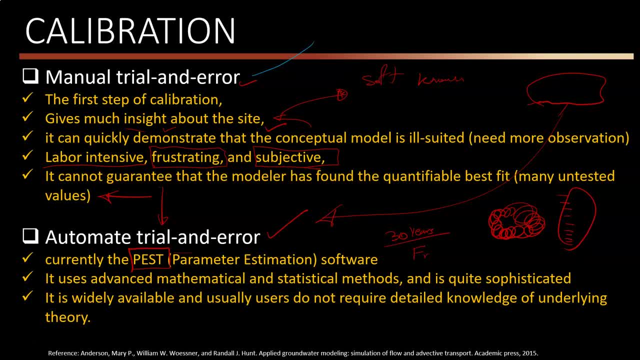 known as PEST, which is freely available so you can go and it's an open source software. Okay, So you can go and actually, if you want, you can go and use this, But But it is not easy to use that, So you need to get trained usually, or study, to be able to use the software. 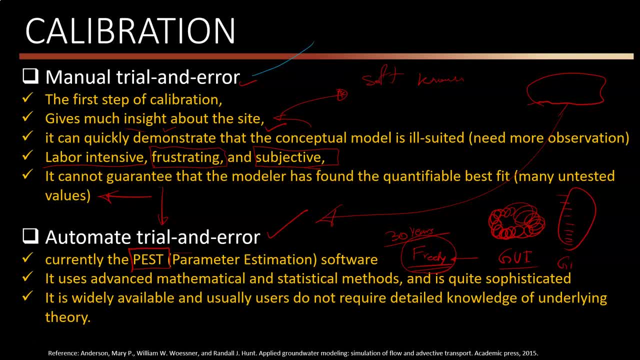 But there are a lot of GUIs and interfaces like GMS, which are actually. they have the PEST feature that you can go and use the interfaces and do the calibration, So you don't need to learn the advanced mathematical and statistical methods or the very detailed knowledge underlying this theory. 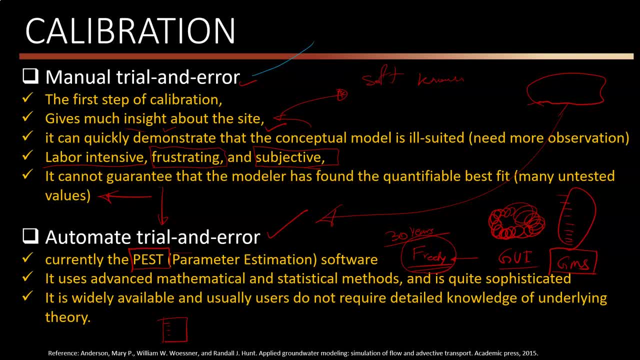 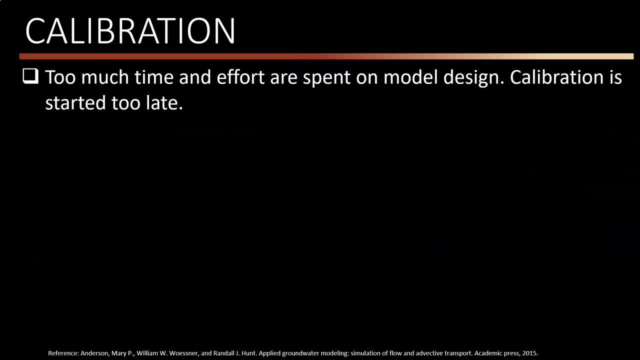 But you need to go and learn how you can apply this PEST method for PEST software or PEST solution to your developed groundwater models. So you're going to solve a few examples, calibration examples, and I want you to go and go and play with and gain some experiences on the calibration. 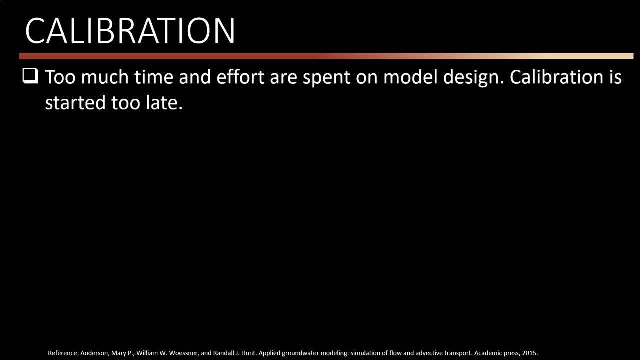 This is as we discussed. the calibration process depends on the experience and the knowledge and it is subjective. So you need to spend time. if you want to be a good groundwater model, You need- you have to be good Calibrator or you have to learn how to calibrate your models. 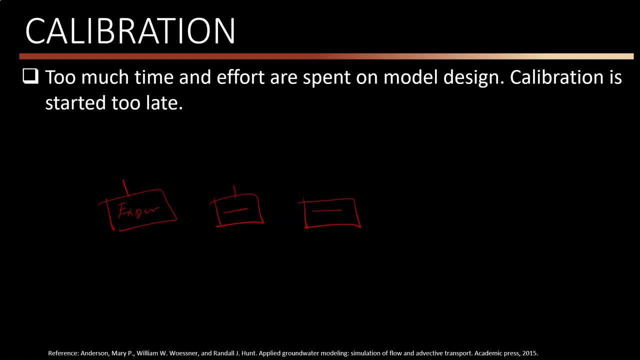 But it is very important- and I've seen this problem a lot- that there are some cases in which they have spent too much time and effort on designing the model And they've just left one month. For example, they spent 11 months on designing, conceptualizing and designing the model. 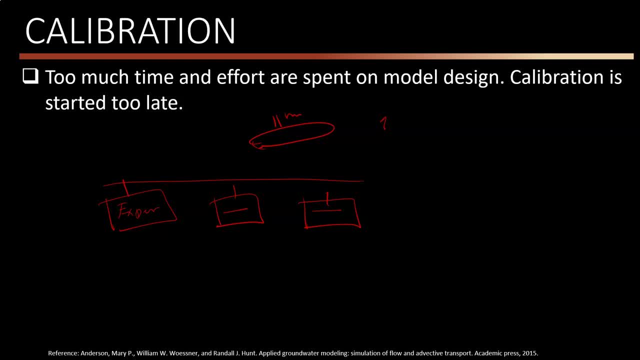 And they've just left one month. For example, they spent 11 months on designing, conceptualizing and designing the model And they've just left one month. And they've just left one month on designing, conceptualizing and designing the model. 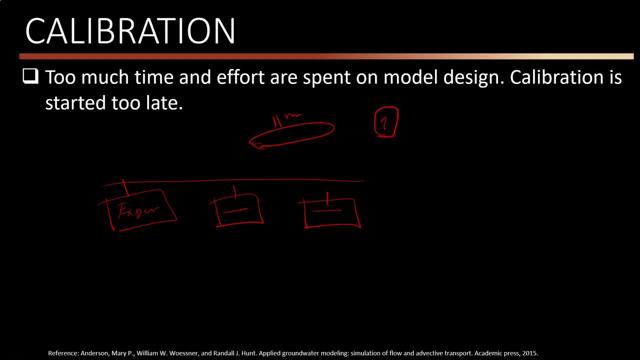 So this is the. So you need to be careful with that That you shouldn't start your calibration model too late, So it takes time. There are a lot of steps that you need to take and this is the way that actually you can show that your calibration model is not disposed to be false. 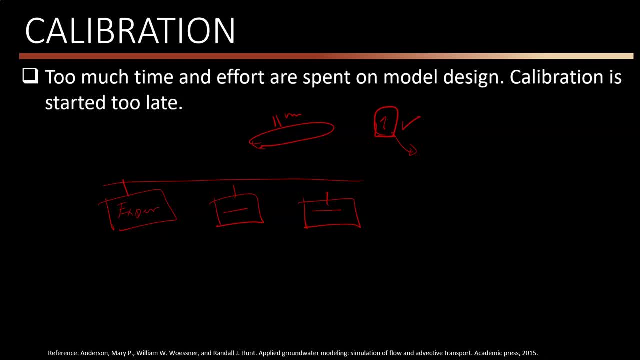 your caliber. your model works right, okay, so this is the only way to go and judge that the model that you have created is right. okay, I will finish this course here, but before doing that, I want to talk about one thing, which is that actually, in this course, we specifically focused on groundwater flow, so we had a 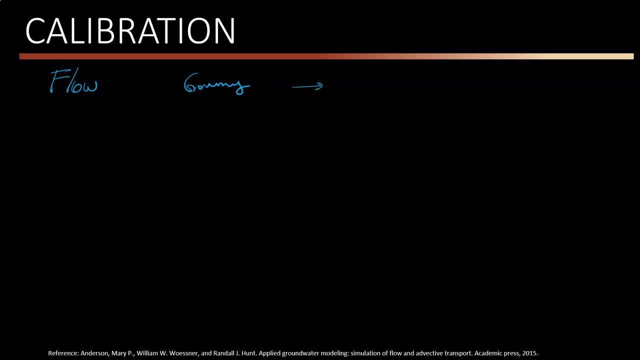 governing equation which went: and if we solve that equation, it will give us H or Phi information at X, Y, Z and T and based on that, we can post, process this information and we can find the gradient or the directions, or flocks and so many other information. 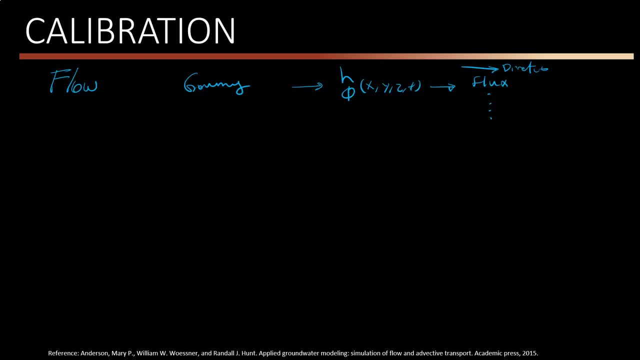 after post processing this information. but groundwater modeling does not stop here. we usually want to find how the head is distributed within the system. we want to find the groundwater head contours because we want to find the groundwater velocity and the direction at each locations. so this is something 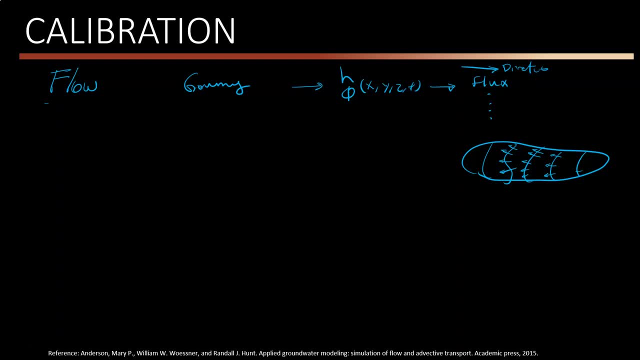 that actually we want to know. but there is another group of problems which we call the contaminants transport. so the contaminant transport has a similar governing equation but its own governing equations, which technically gets the flux flow information from the groundwater flow model and use it and use those. 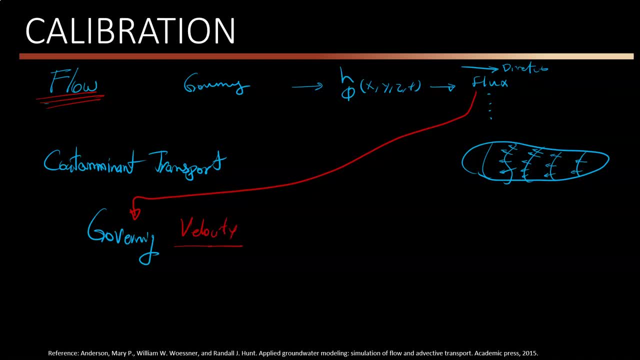 information, technically the velocity information, and they go and solve how the contaminant changes at each x, y, z and t. So we don't talk. we didn't talk about the contaminant transport models. in other class of mine we specifically talk about the governing equations of the contaminant transport and we 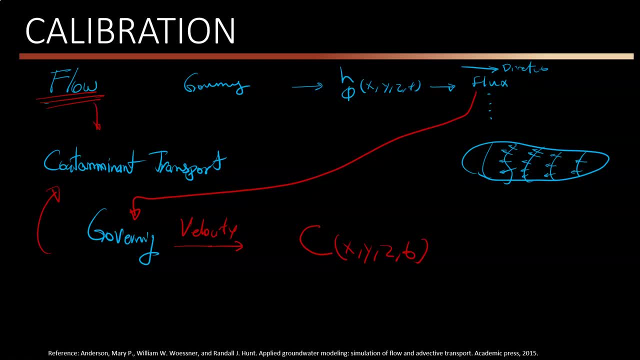 learn how we use the information here and apply it here to see how contaminants, how the plumes, will move within the system. But this is a very similar process. so the process of the contaminant transport and groundwater flow is very similar. It has its own governing. 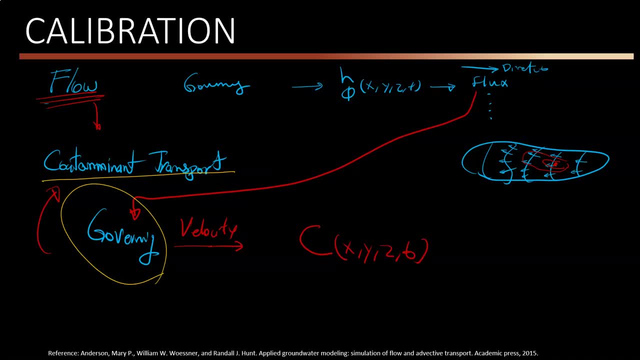 equation. there are some methods and softwares and packages like MT3D or RT3D that actually we again- we discuss these in other class- but they have their own packages and you need to do the find this and eventually you need to go and find the calibration, actually do the calibration. so the process is: 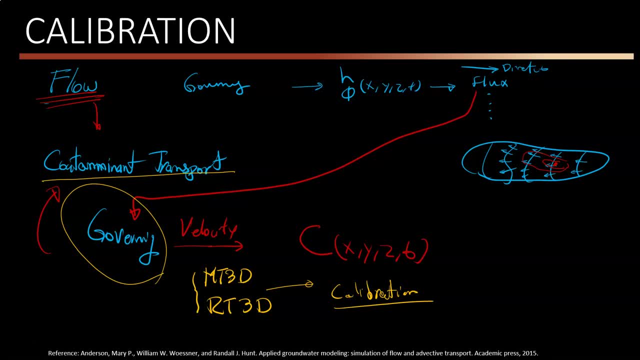 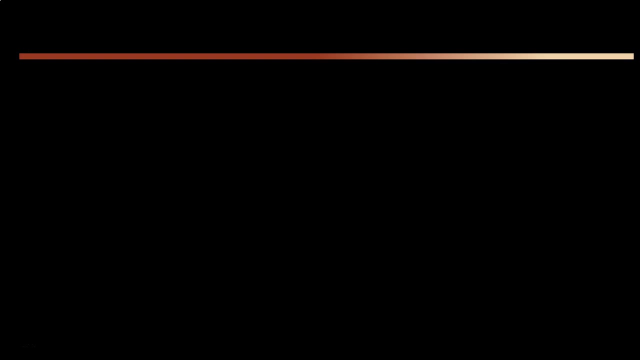 pretty much the same, but with different groundwater, but with different governing equations technically. so I believe that actually, by the knowledge that you've gained by taking this class, you can go and learn and practice the contaminant transport modeling as well. I have you. I hope you've enjoyed this course and you've learned useful techniques and skills to 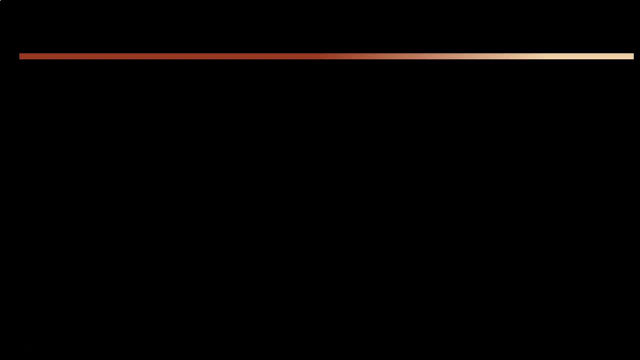 become good groundwater model in the future and probably build your career on. if you have any questions, you can send me an email, as you did before, or you can stop by my office. we can work on your questions and I hope that you've learned to mine. the main objectives or the main goal of mine was: 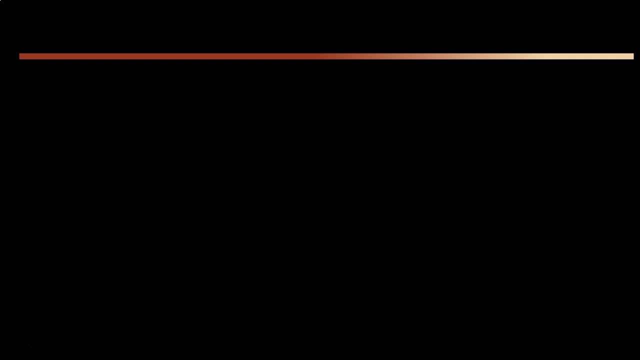 to teach you in a plain and simple language how, what is the flow, the philosophy of groundwater modeling and how you can create an accurate and reliable groundwater models. and I hope that actually you've learned new things, but there are very good sources around that you can go and.